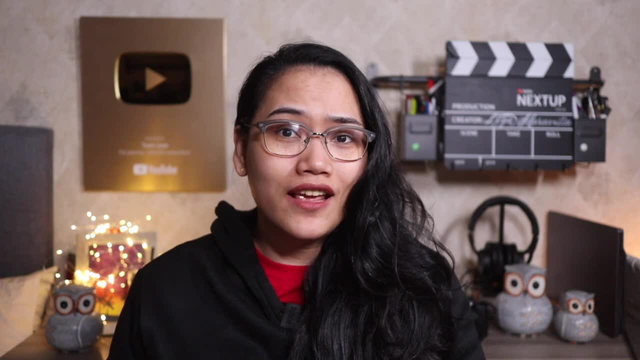 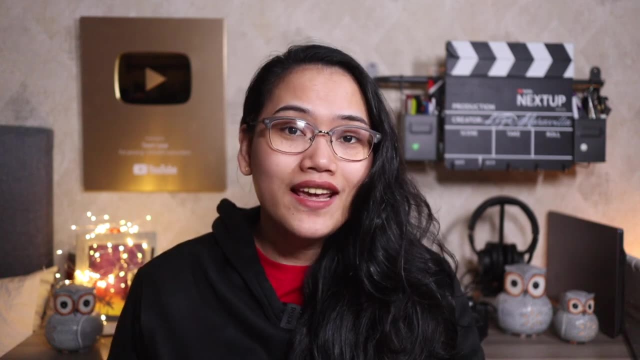 Now, like I said in the intro earlier, we're going to talk about the rules for 10,, 11, and 12.. If you haven't watched our video discussions on 3,, 4,, 5,, 6,, 7,, 8, and 9,, 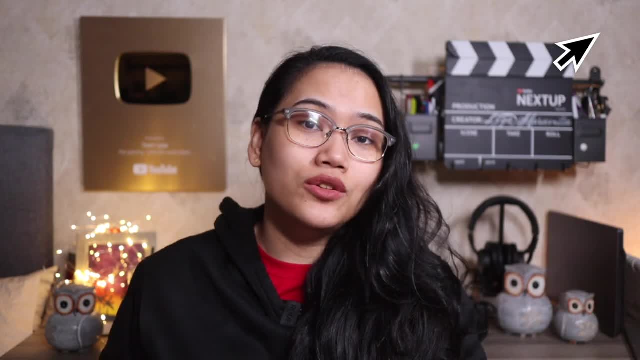 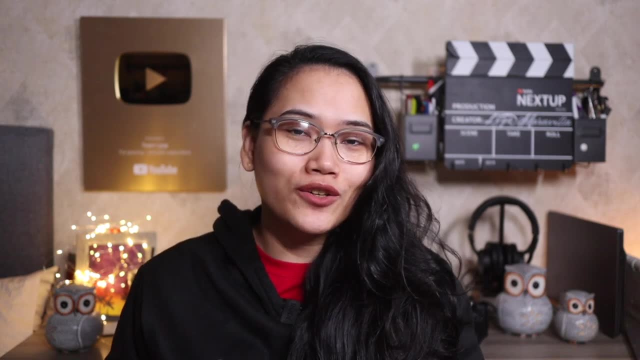 the links to those videos will be right here on the i button if you're watching on YouTube or in the description box below. Okay, you can go ahead and watch those first and then go back to it, Because these are the rules. These are a little bit, just a little bit challenging than the rest. 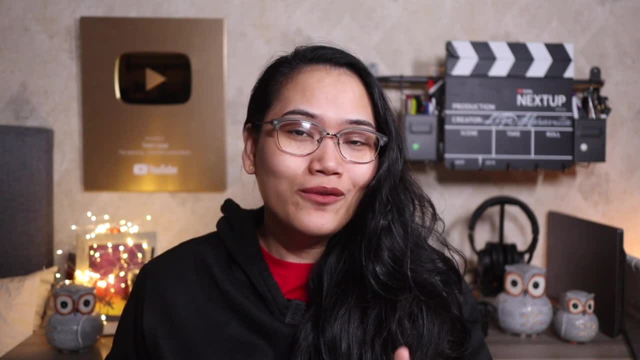 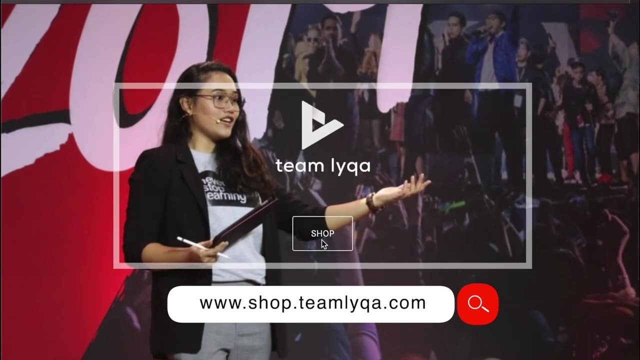 All right, And it will also require some of those digits which we'll talk about later. But before you do that, just a quick little plug If you want to help support this channel and our cause to democratize the education of the Philippines. 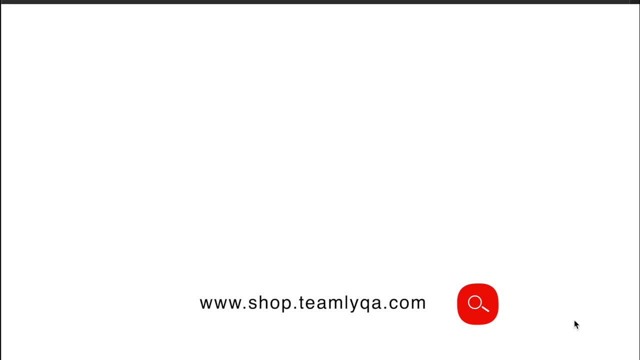 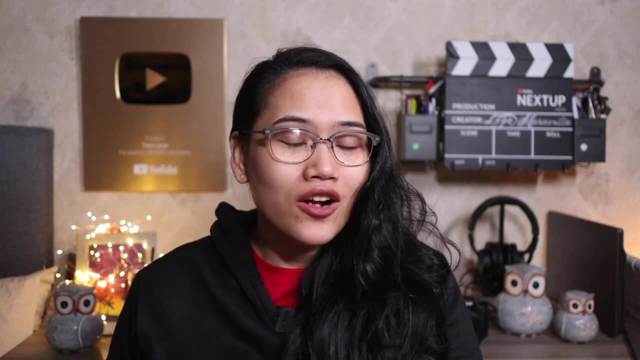 one way that you can do that is through buying our merch. You can visit shopteamlaikacom to buy our hoodies, shirts, caps, mugs and more, Or you can drop by our stall or our box on box Green Hills. 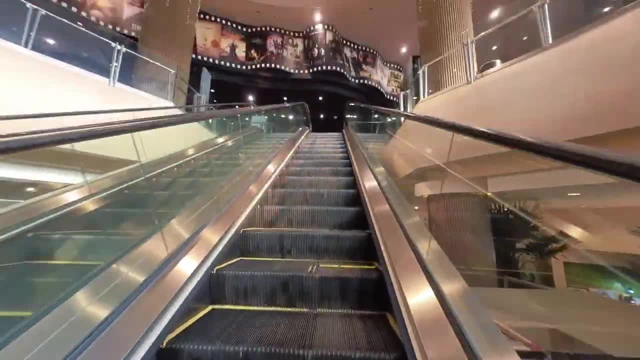 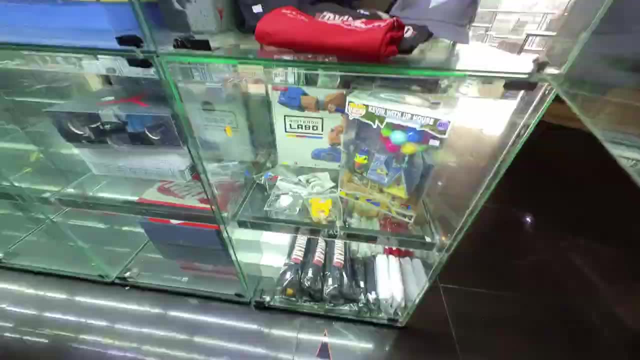 It's located in Promenade Hall in Green Hills. You can just turn right when you go up to the escalator in the cinema And you can find it on box 75,. all right, And now that we have that out of the way, I'm going to switch over to my tablet. 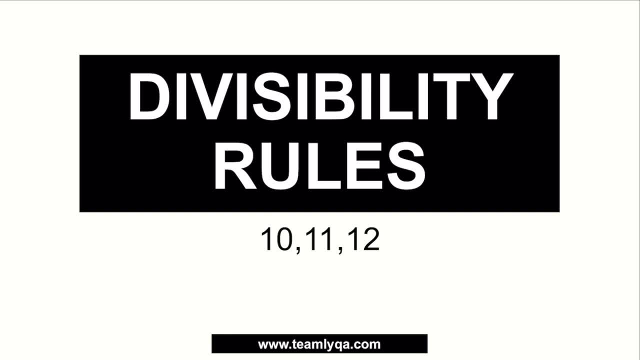 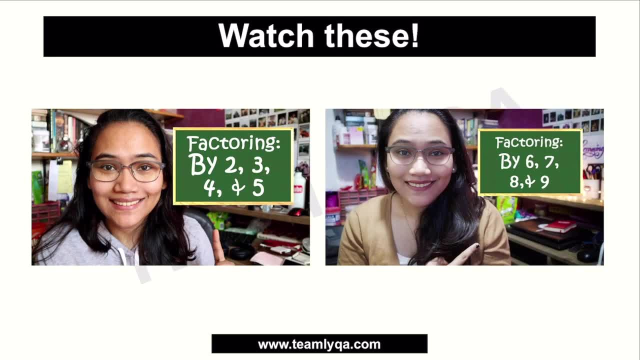 I'll see you in a bit. All right, this is our lesson on the visibility rules. We're going to talk about the rules on number 10, 11, and 12,. okay, And I'll also repeat that. please watch the first two videos. 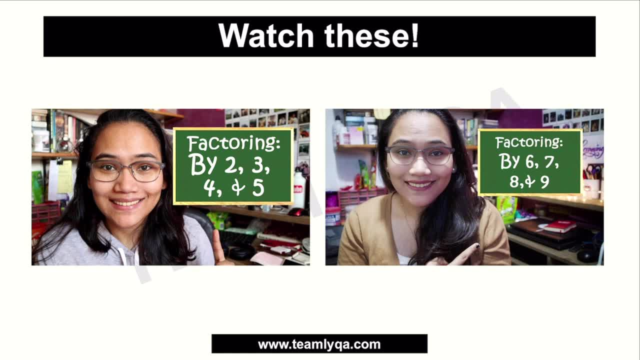 because we're going to use the other concepts in this lesson. okay, So if you haven't watched it yet, the links are there. There's an i button if you're watching on YouTube or in the description box below. These are older videos, but that's okay, even if the quality isn't the same. 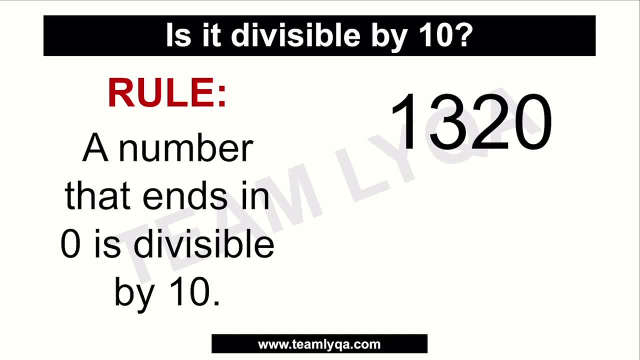 The lesson is important there. okay, We're going to start with number 10.. This is the simpler part. The rule is that a number that ends in zero is divisible by 10.. So if we have a number like 1320, because its last digit is zero, 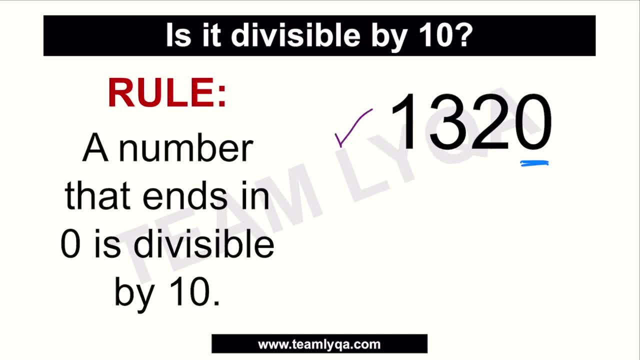 it means this is divisible by 10.. Okay, Now, why is that? A simple illustration would work like this, right, If we multiply a number, for example 23.. If we multiply it by 10, what we're doing is we're going to put a zero at the end of 23.. 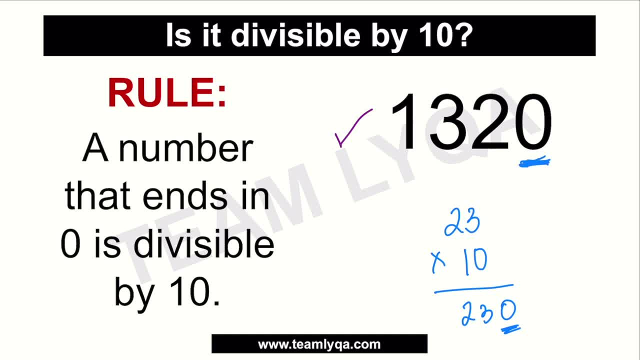 Okay, So again, any number whose last digit is zero is divisible by 10.. Okay, So that's very easy. Next, we're going to use the same number, 1320.. Let's see if we can figure it out. 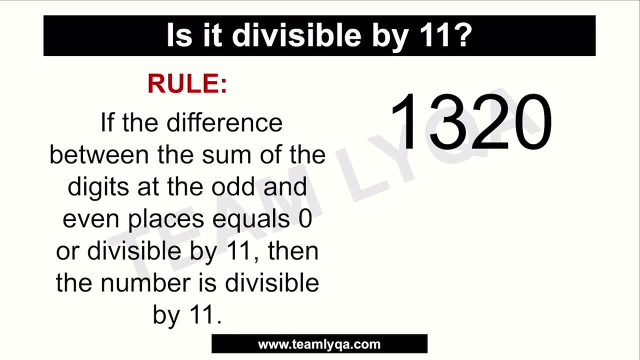 Let's figure out if it's divisible by 11.. Now the rule for 11 is a little more detailed, but bear with me, You can do it. The rule is that if the difference between the sum of the digits at the odd and even 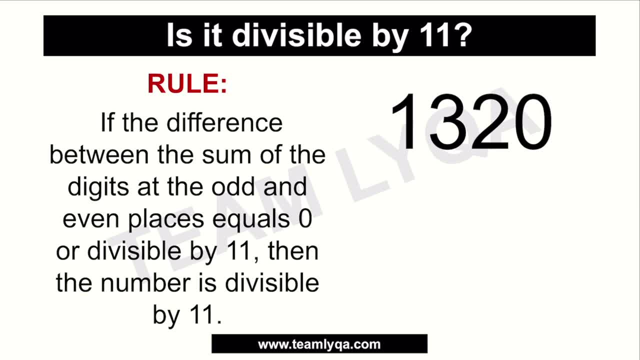 places equals zero or is divisible by 11, then the number is divisible by 11.. Now I know the instructions are long, but I'll show you how to do it. Okay, We're going to start from left to right. We're going to mark the ones at the odd and even places. 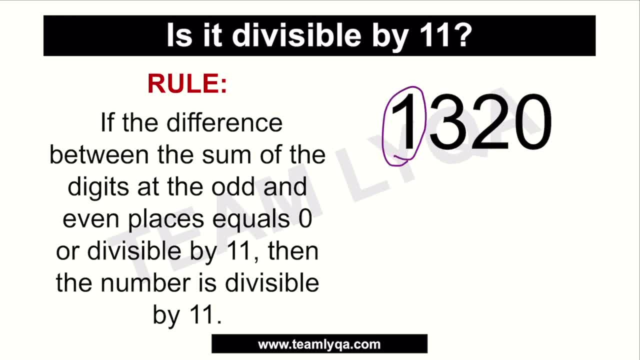 What does that mean? You have 1, then you'll skip, and 2.. Okay, These two are at the odd places, So what we're going to do is: 1 plus 2 is equal to 3.. Okay, We have that. 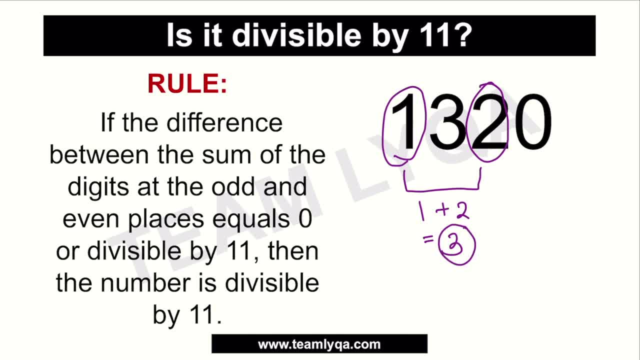 That's the sum of the digits at the odd places. Now let's go to the even. You have 3 and 0.. Now what does that mean? 3 and 0.. 3 plus 0 is equal to 3.. 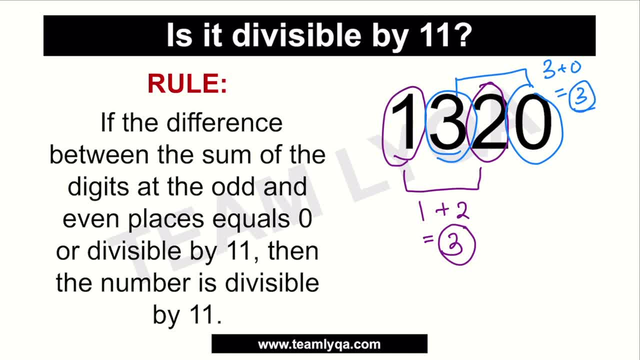 So that's the sum of the digits at the even places, Okay, Or actually you can call it interchangeable. It depends on where you started, If it's at the right or left. Okay, Now what we're going to do next is just to subtract 3 from 3.. 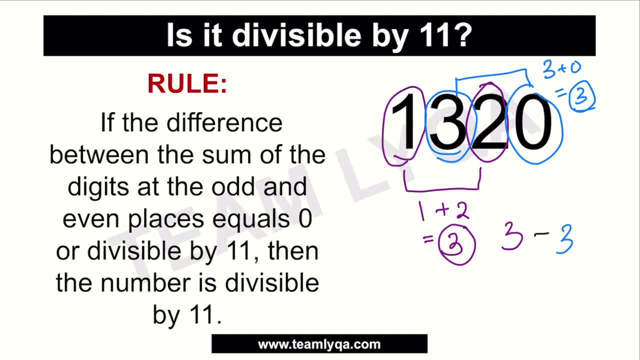 Okay, So 3 minus 3.. Okay, This is it? This 3 is it This, 3 is it? Now, if their difference is 0 or 11, it means that the number is divisible by 11.. Now, 3 minus 3 is 0,, which means that 1,320 is divisible by 11.. 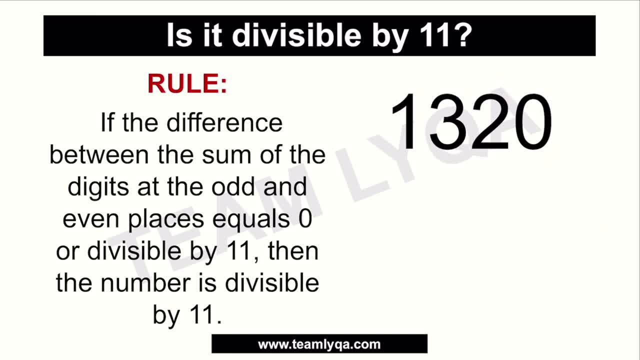 Okay Now how are we going to check this? If you want to check, we can just divide this really quickly by 11.. Okay, So 13 divided by 11 is 1. 11.. Let's just subtract that. 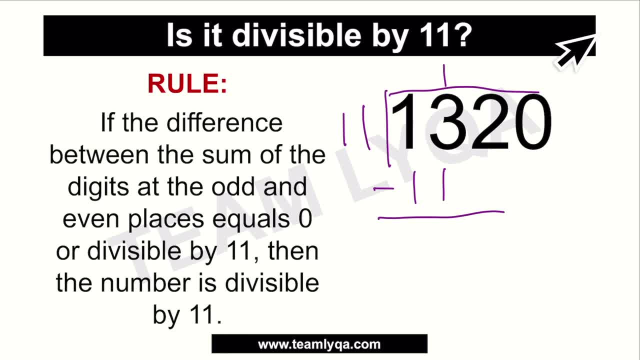 This is just long division. If I forgot, I will also link the lesson in the upper part of the video. in long division This is going to be 2.. Let's subtract that 22.. 13 divided by 11 is 2.. 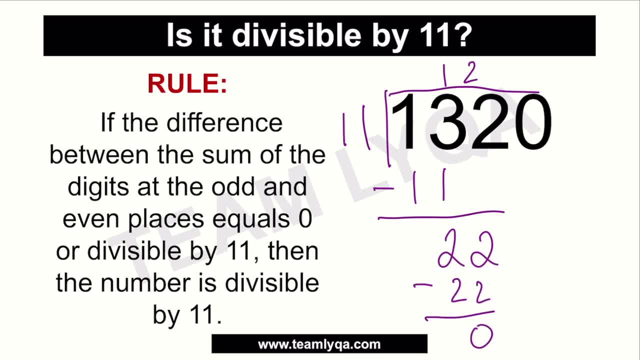 2 times 11 is 22.. If we subtract this, it's already 0.. So it means that we're just going to put 0 at the end. So, yes, there's no remainder. It means that it's really divisible by 11.. 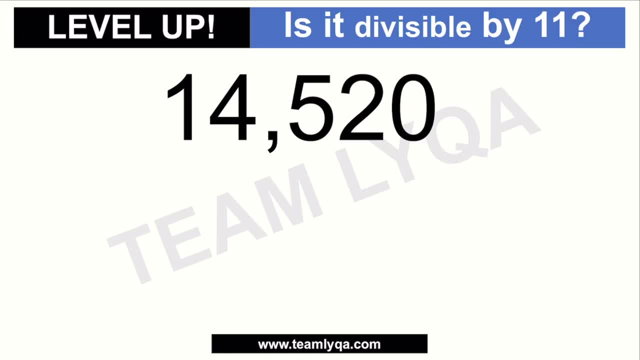 Okay Now, because of the 3 numbers that we're talking about now, 11 is the most tricky. Here's a leveled up example: Is this number 14,520, divisible by 11?? Okay, I'll give you time. 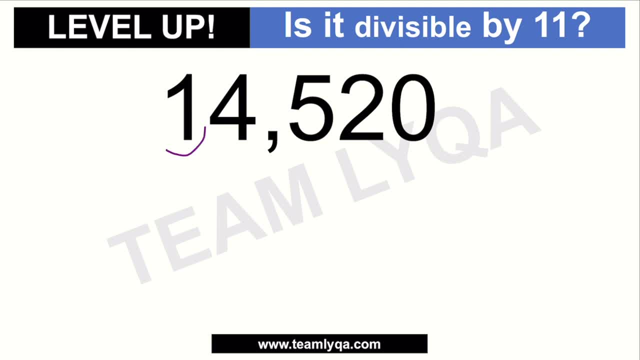 Alright, let's see how you did. So we're going to do the same thing. Let's take 1, skip 5, and 0. If we combine these, 1 plus 5 plus 0, is 6.. 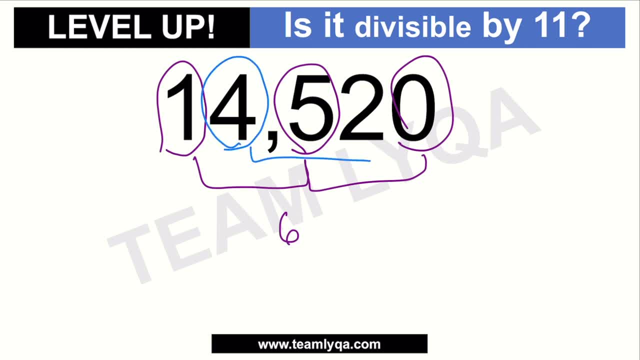 Next we're going to do the remaining numbers: 4,, skip and 2.. 4 plus 2 is 6.. Now, if we subtract that, what we'll get is 0. Which means that 14,520 is divisible by 11.. 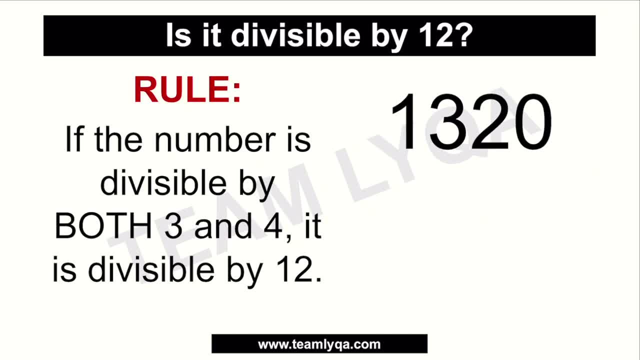 Okay, Next we're going to look at 12.. Now the number 12, to know if a number, especially a big number, is divisible by 12, you need to check if it's divisible by both 3 and 4.. 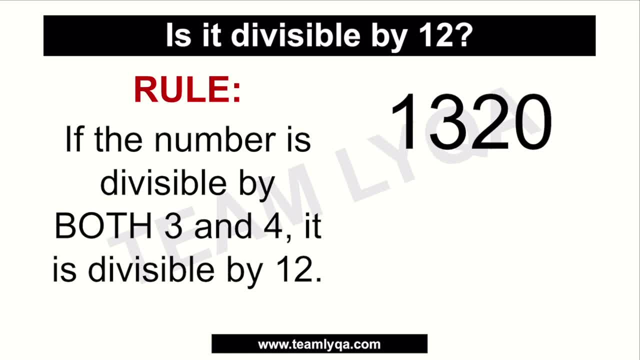 Okay, Now if it's divisible by 3 and 4,, it means that it's divisible by 12.. Now, how do we do that? Let's start with 3.. Now, if the number is divisible by 3, and again, it's there in our first video, which. 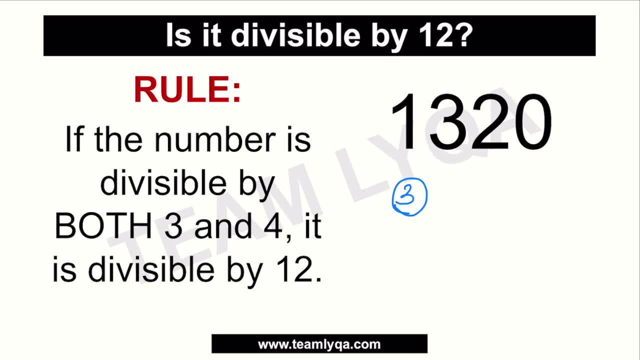 is also linked at the top of the i button. what we're going to do is add the digits, So 1 plus 3 plus 2 plus 0.. 1 plus 3 is 4, plus 2 is 6, plus 0 is still 6.. 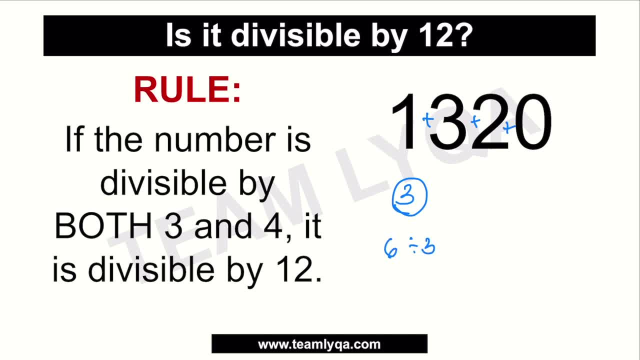 And what is that sum? If you can divide it by 2,, it's 6.. If you can divide it by 3, and the answer is complete, so 6 divided by 3 is 2,, it means that it's divisible by 3.. 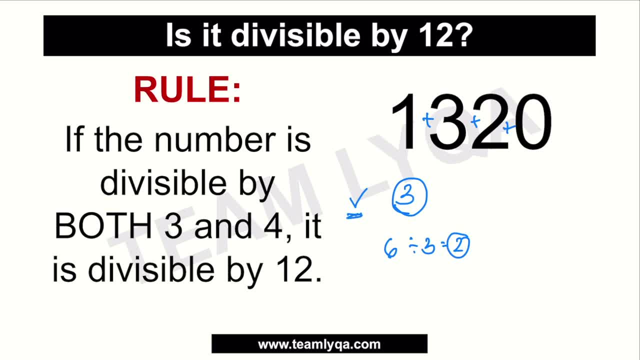 We're now okay with 3.. Now, how about 4? Divisibility in 4,. one of the things we need to do is look at the last two digits. Now, why is that? Because the last two digits will determine if this number is divisible by 4.. 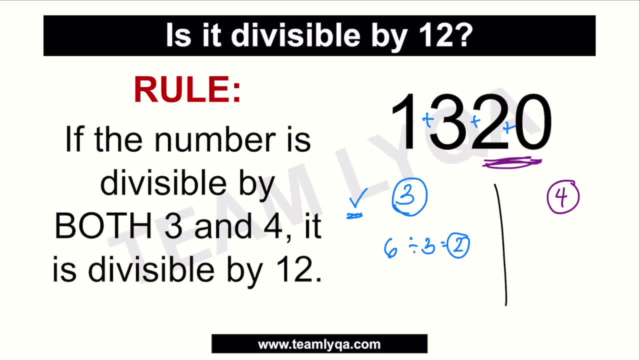 100 is divisible by 4.. 100 is divisible by 4.. So, since all the hundreds are made up of thousands, as long as it's over there, it's divisible by 4.. So 1300 is divisible by 4.. 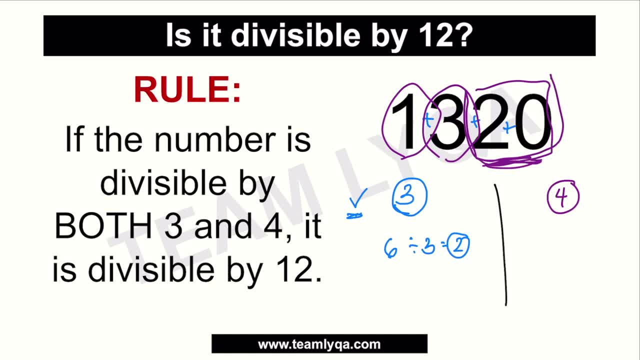 But to find out what the whole number is, we'll look at the last two digits Now. because 20 can be divided by 4, it will result in 5,, which means it's divisible by 4.. And because it's okay with 3,, it's okay with 4,, which means this number- 1320, is divisible. 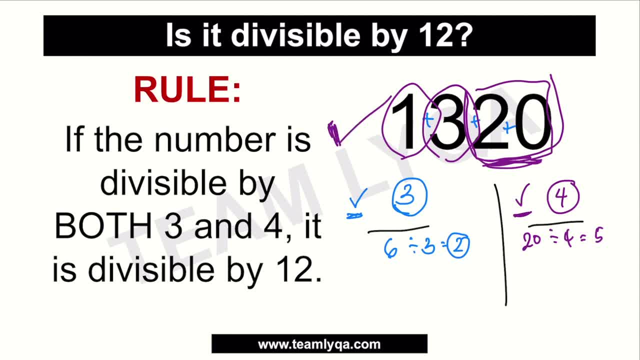 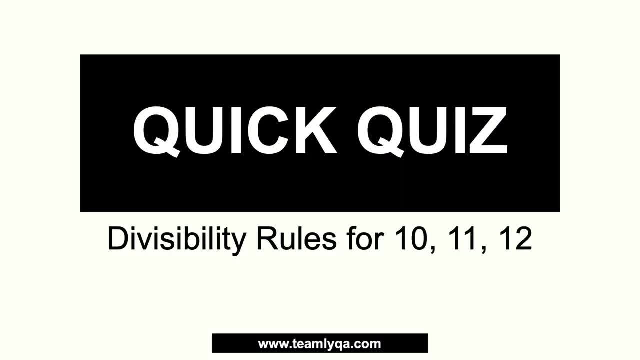 by 12.. Okay, So again, that's our rule. It should be divisible by 3 and 4. It can't be just one. Alright, now it's time for your quick quiz. If you're ready, with your pen and paper, all you're going to do is to check if this number 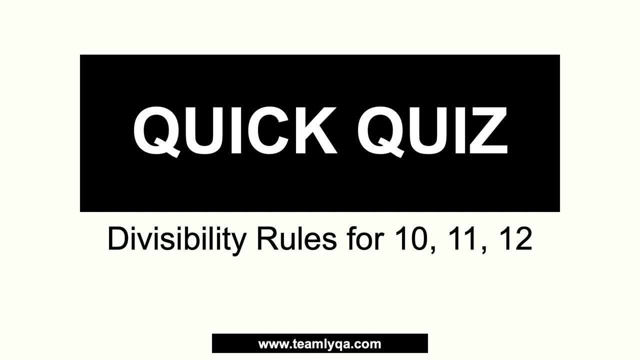 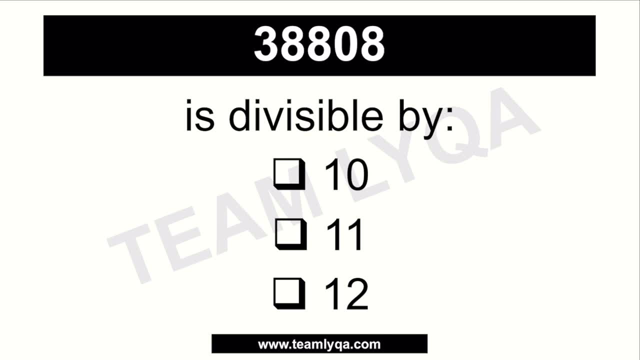 is divisible by 10,, 11, and 12. And your timer starts now. Here's what you're going to do: to find out if this number is divisible by 12.. The con какую you're going to do is to take the first 1982 numbers and just minus the 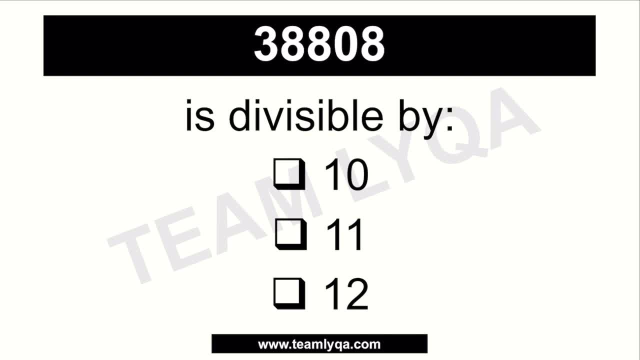 values of this number for its value. We're going to do this in the middle position so that you can match, And you're going to do a cliché similar to the last Claus rule. So we'll just go for the slops. 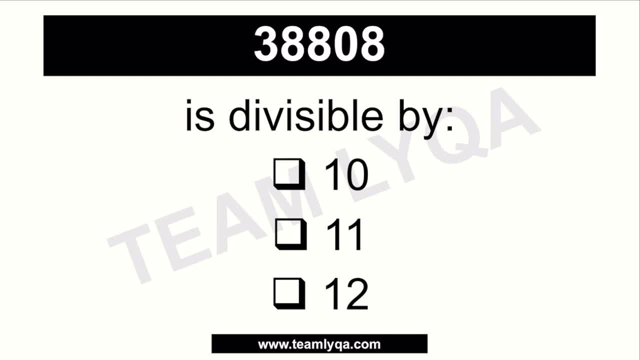 Glossy zones in 2015. it means what came from a given tile. All right, let's see how you did So. our number is 38,808.. For us to know if it's divisible by 10,, the last number is 0,. 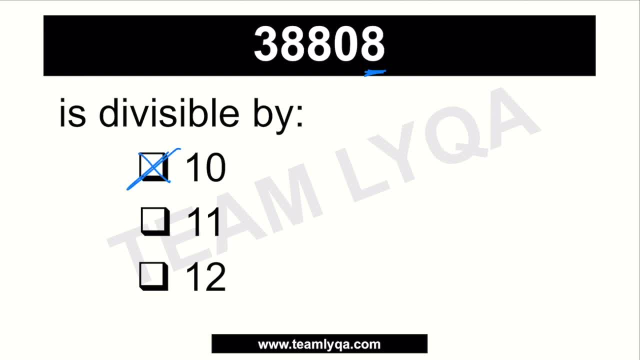 which is not the case here, Which means it's not divisible by 10.. Okay, Now to find out if it's divisible by 11, what we need to do is we'll get the odd places of numbers and the even places of numbers. 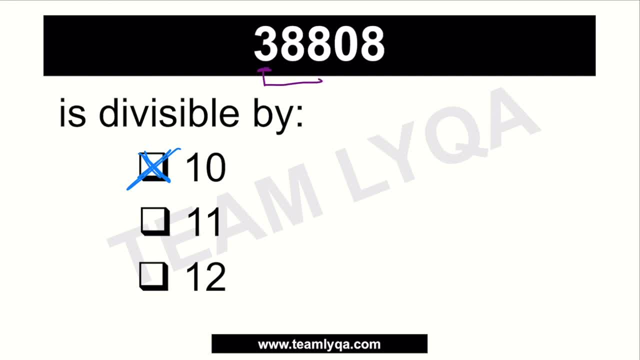 So let's start here with 3,, 8, and another 8.. Now, 3 plus 8 is 11, plus 8 is 19.. Okay, Now let's get the even places. You have 8 and 0.. 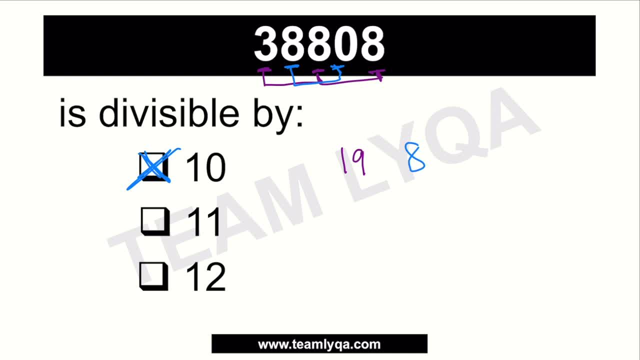 8 plus 0 is 8.. Now let's just subtract that 19 minus 8 is equal to 11.. Now let's say if it's 11 or 0, and because it's 11, 38,808 is divisible by 11.. 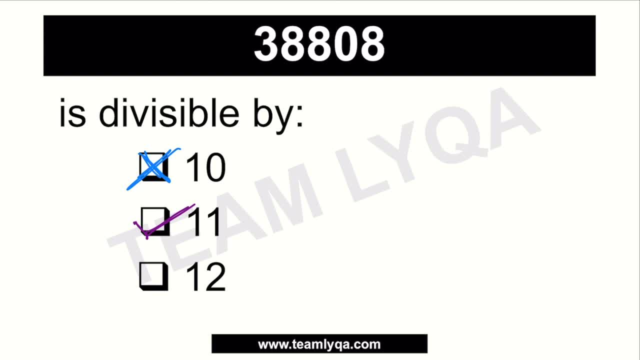 Let's check that. Next we're going to look at 12.. Now let's say it needs to be in 3 and 4.. Okay, Let's start with 3.. We'll add them all. So 3 plus 8 is 11, plus 8 is 19,. plus 0 is still 19.. 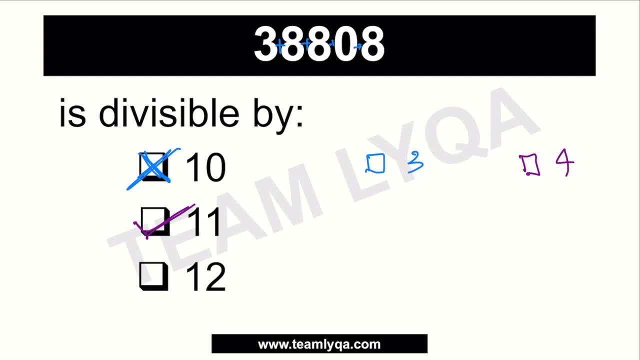 Okay, But let's also respect that This is turning first right. 12 plus 7 is 1, so 3 plus 7 is 18.. We're literally it's already 14,. it's already in 3,. 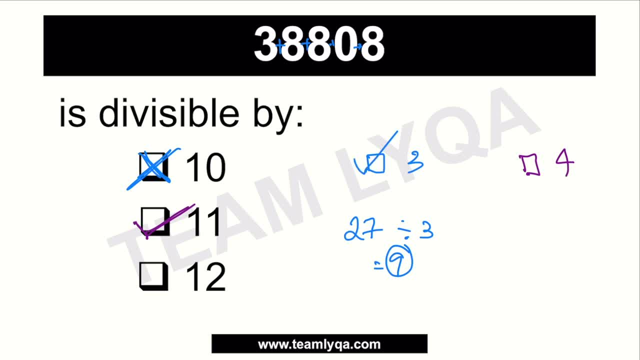 but here it's being公. Now 8 plus 1 is previously in 3. So we separate 2 and 3.. Now 27 plus 9 is 26.. You can see here how much time does it have to go through. 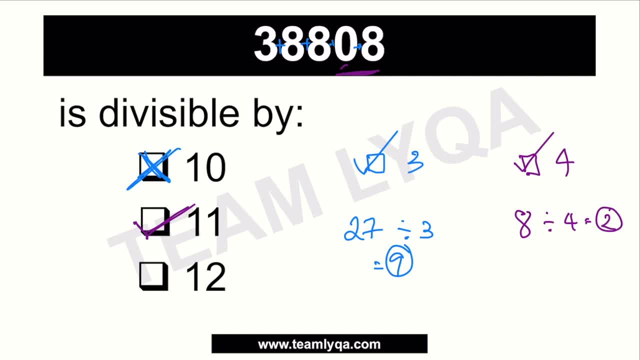 You have to think about how long is this going? It has 8 days. the Senate will scale in numbers. What will they see if it is 21 years old? yan yung sagot natin: Hindi sya pwede sa 10, pero pwede sya sa 11 and 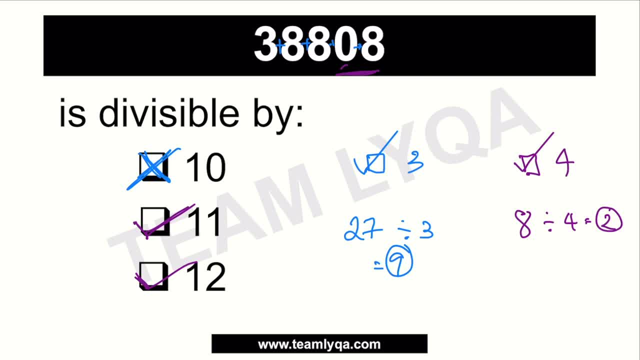 12. Now yung mga nagtatanong: isan ko ito gagamitin? Sa totoo lang, marami syang applications Pwede nyo syang gamitin kapag hinahanap nyo yung square root. 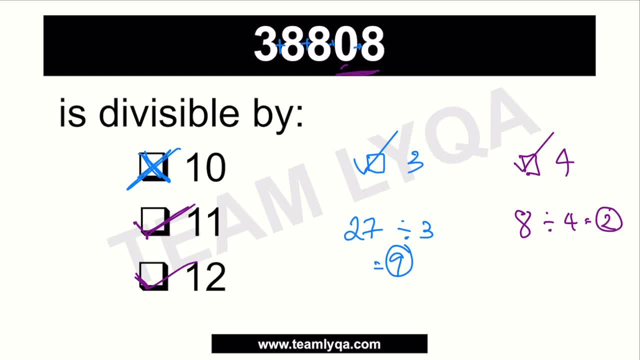 Pwede nyo yung gamitin pag nagfa-factor na kayo. Pwede nyo syang gamitin kapag nagdi-divide kayo or nagbumultiply ng mga fractions, para alam nyo kung ano yung ika-cancel. So again, 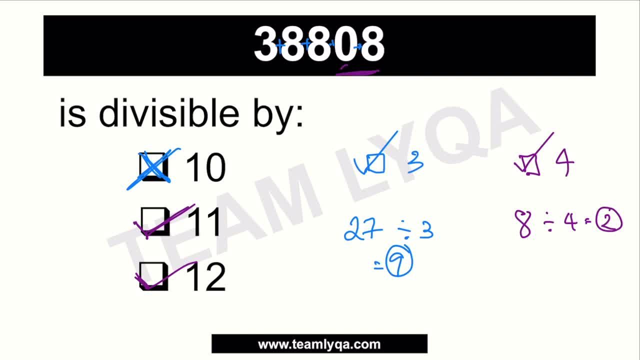 marami itong applications and I'm hoping makatulong ito sa inyo para bumilis kayo sa math. Okay, Alright, now I hope you got this all correctly. If you didn't, that's okay, I'll be posting. 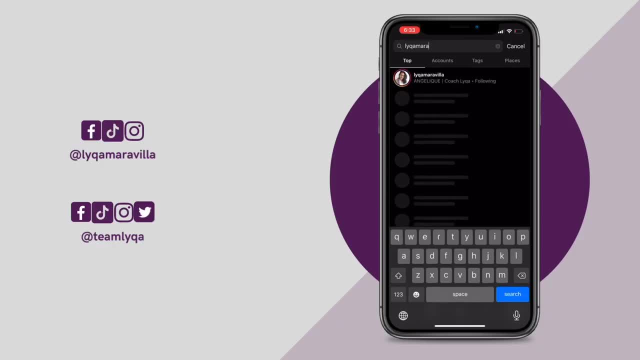 more questions on my Instagram account. So if you don't follow me yet, you can follow me at Laika Maravillo on Instagram for the new quick quiz questions na pinapost ko sa Instagram story. May function kasi doon na quiz kaya.